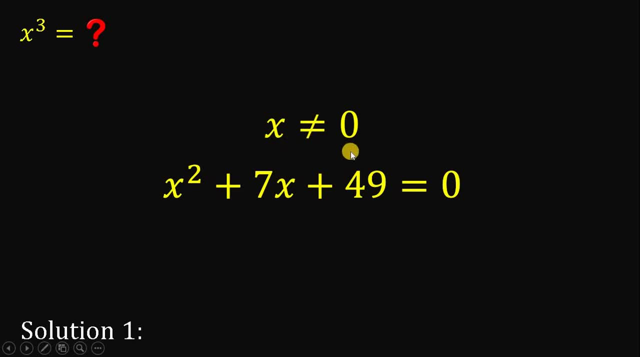 Now, this is safe because we know that x is not equal to 0.. But before that, let's put this equation right here. Maybe we will use this equation later on. Now again, let's multiply both sides by x. Again, this is safe because we know x is not equal to 0.. 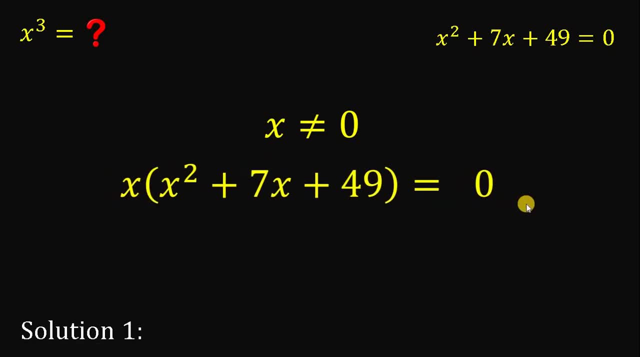 On the right hand side, x times 0 is just 0.. And on the left hand side, x multiplied by 0 is 0. So x multiplied by x squared plus 7x plus 49 will give us x cubed plus 7x squared plus 49x. 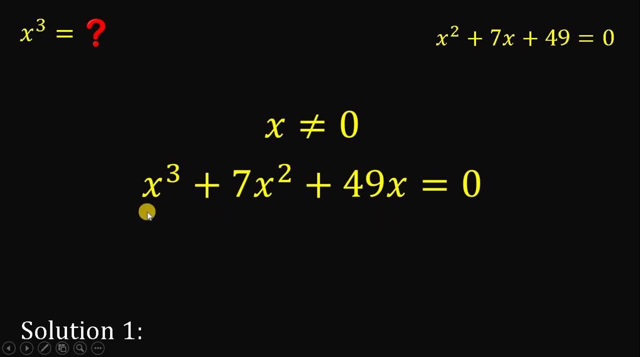 Now what we're going to do here is to isolate x cubed, So rearrange some terms a little bit. This will give us x cubed equals negative 7x squared minus 49x. Now let's factor out negative 7, because we know 49 is just 7 times 7.. 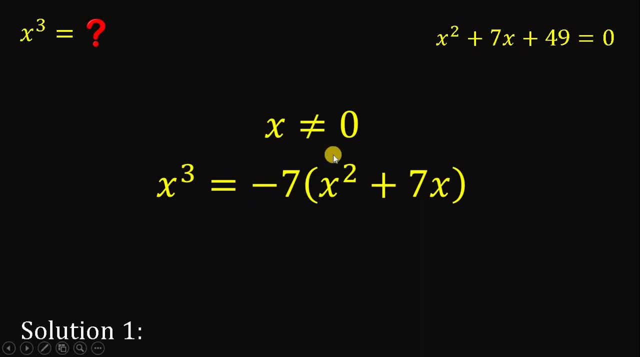 So let's factor out negative 7.. This will give us negative 7 multiplied by x squared plus 7x. Now, on the given equation a while ago, x squared plus 7x plus 49 equals 0.. If we subtract 49 on both sides, this will give us x squared plus 7x equals negative 49.. 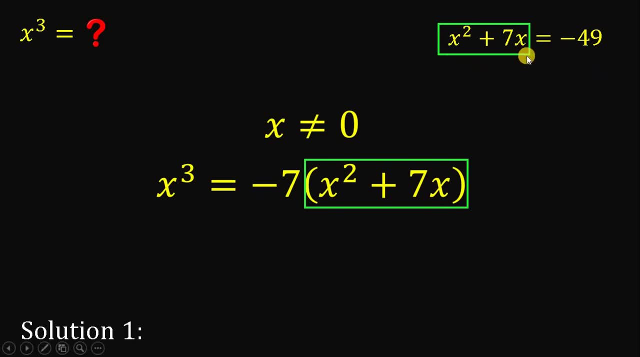 Now look at this. We have the same expression, x squared plus 7x, And we know it is equivalent to negative 49. Therefore, we can replace this expression by negative 49.. So we have now: x cubed is equal to negative 7 times negative 49.. 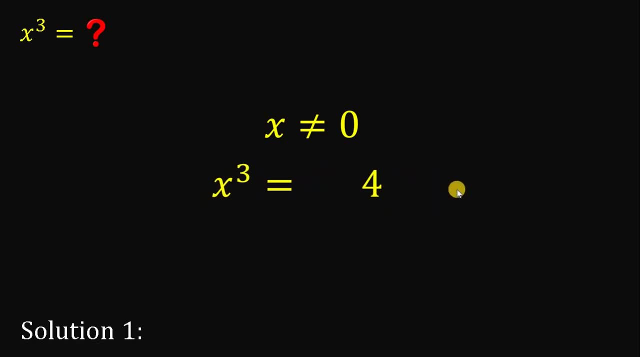 And negative 7 times negative, 49 is simply 343.. Therefore, using our first solution, we get that x cubed is simply equal to 343.. Now let's have our second solution. This is much easier than the first. Now, first thing to notice is, in this equation, x is not equal to 7.. 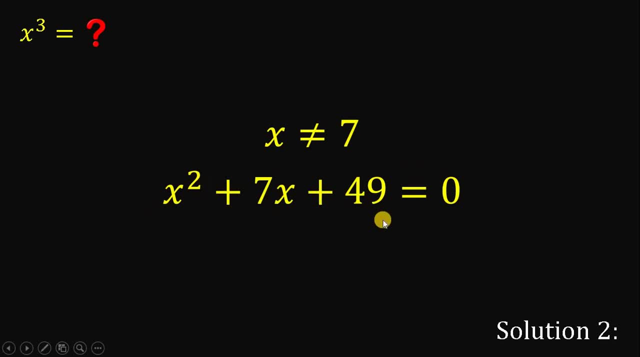 Because if we replace x equal to 7, the left-hand side is not equal to 0. So if x is not equal to 7, x minus 7 is not equal to 0. So we can multiply both sides by x minus 7..